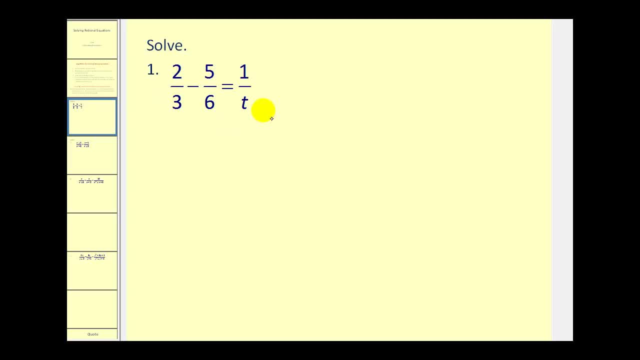 the LCD or least common denominator. This problem, without factoring the denominators. The LCD in this case would be 6T. That means we're going to multiply both sides of the equation by 6T, or 6T over 1.. Well, what I'm going to do is I'm going to multiply every single term by 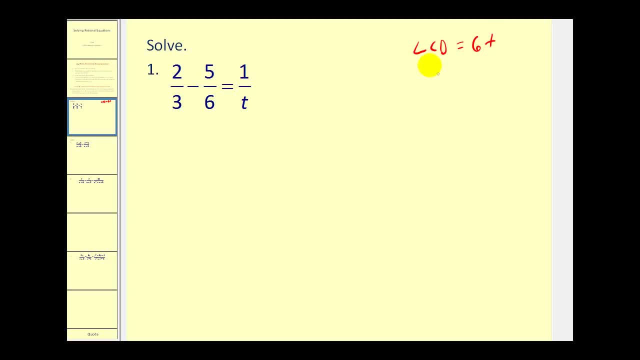 6T over 1, because it makes simplifying those products a lot easier. This is what I mean by that. I'll take each of these terms and multiply by 6T over 1.. Now we'll simplify each of these products. This was changed to a 1.. This was changed to a 2.. 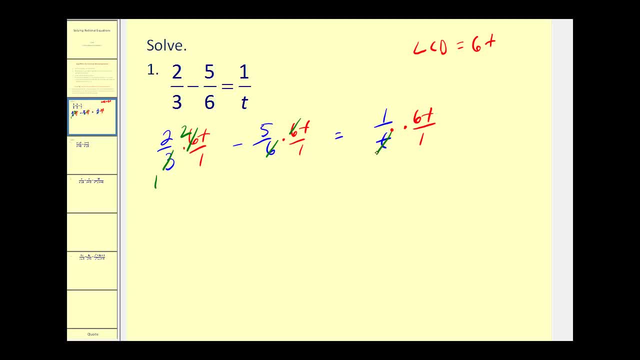 Here the 6's simplify out And here the T's simplified out. Let's see what remains. Here we have 2 times 2 times T, all over 1.. That's 4T. Here we have 5 times T, So we have: 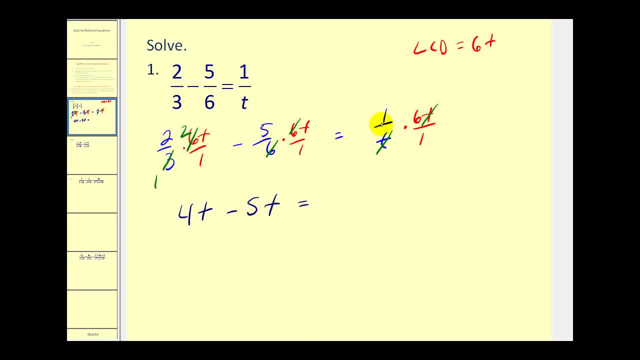 minus 5T, And here we have 1 times 6 all over 1, which is just 6.. So we've created an equation that is much easier to solve than the original rational equation. So here we can combine our like terms. This would be: negative T equals 6.. You can think of this as: 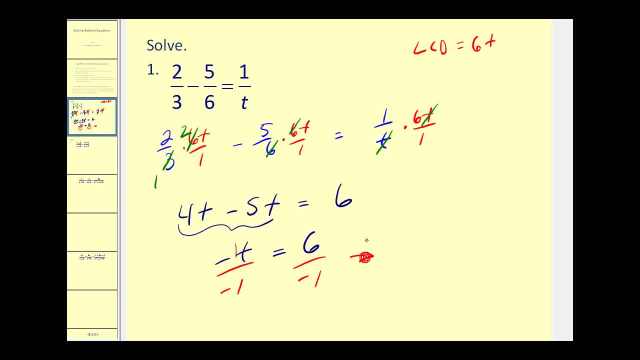 negative 1T divided by negative 1.. So we have T equals negative 6.. Let's go ahead and try another. Even though this is a proportion, I'm going to go ahead and follow the rules outlined in this video. We can see the LCD would be the product. 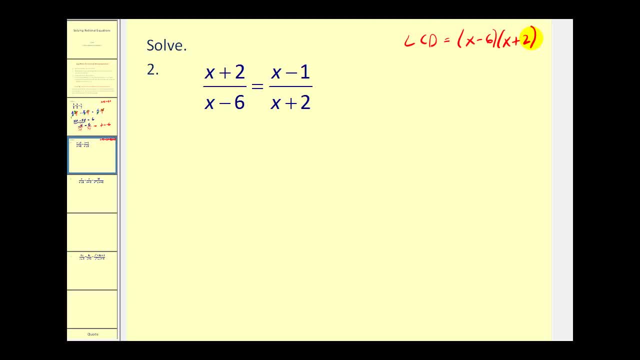 of these two denominators. So we'll multiply both sides of the equation by this product over 1.. So notice in red: we've multiplied both sides of the equation by x minus 6 times x plus 2, all over 1.. Now let's go ahead and simplify. Notice: we have a common factor of x minus 6 here. So 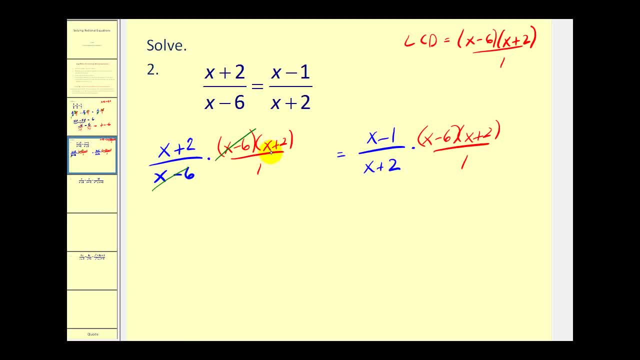 we're left with x plus 2 times x plus 2.. Must equal Over. here. we have an x plus 2 on top, x plus 2 on the bottom, So we're left with x minus 1 times x minus 6.. So the fractions are gone. but 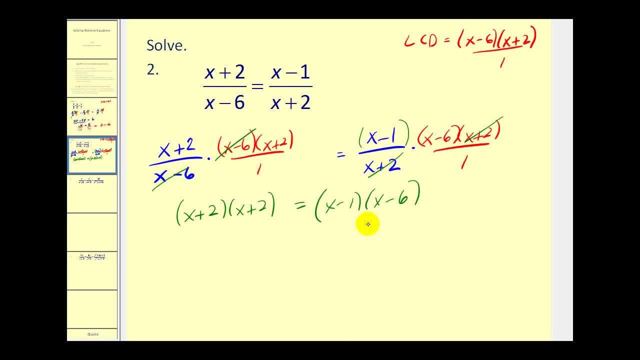 now we have to multiply this out and solve for x, So we're going to have to foil both sides. here We'll have x squared plus 2x plus 2x, That's plus 4x plus 4 equals. here we have x squared minus 6x minus 1x, that's. 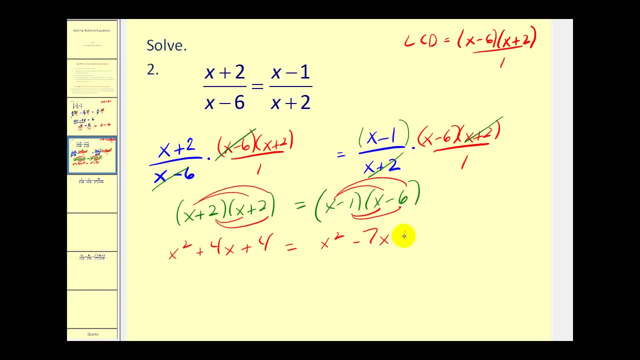 minus seven, x plus six. Now we're lucky here, because if we subtract x squared on both sides, the x squared term goes out, so we do have a linear equation left. Let's go ahead and add seven x on both sides, We would have 11. x plus four equals six. 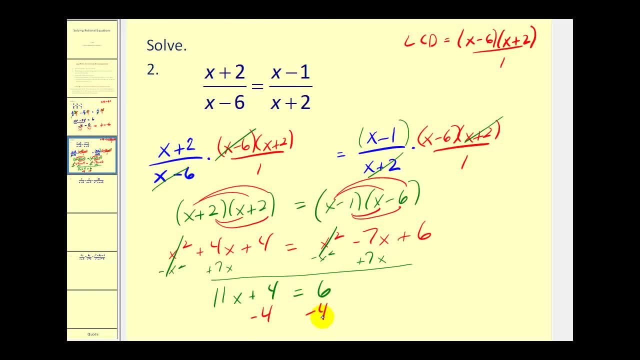 Now we'll subtract four on both sides. I'm running out of room here. Let's go ahead and bring this up here. We would have 11 x equals two. divided by 11 x equals 2 11ths. Remember the guidelines did say: check our solutions. 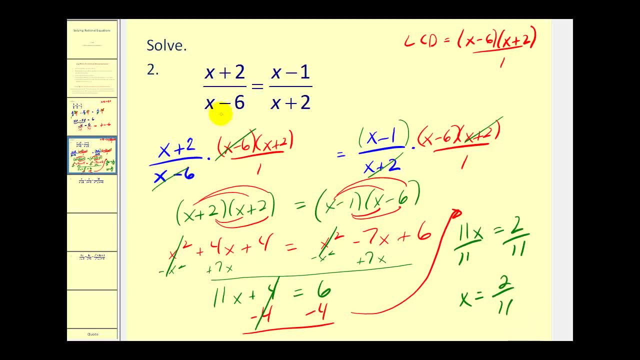 but really what we're checking for is x can never equal six or negative two, because it would make these denominators equal to zero and therefore undefined. So x equals 2 11ths. we'll assume, we'll check. However, let's go ahead and check this one. 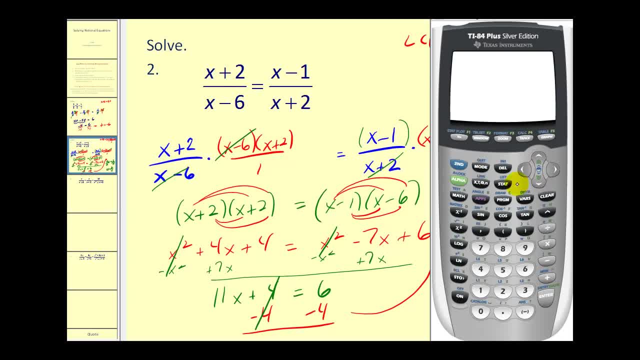 on the graphing calculator. First let's check: two divided by 11 in decimal form is .18. repeating, Let's go to y equals. let's type the left side in y one and the right side in y two. Let's go ahead and press graph. 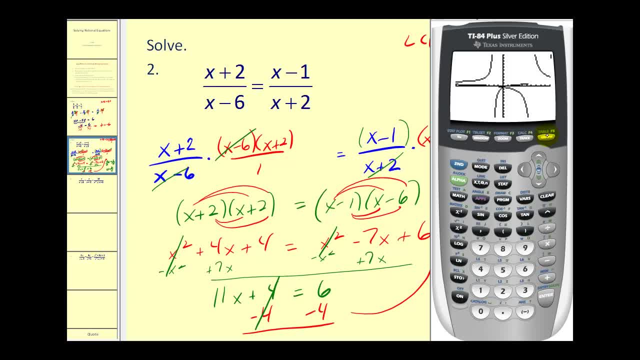 Again, we're looking for the x coordinate of the point of intersection And it looks like it's somewhere right in here. Let's go ahead and calculate it. Second trace, option five: Press enter, enter, enter. And this does verify our solution as two 11ths. 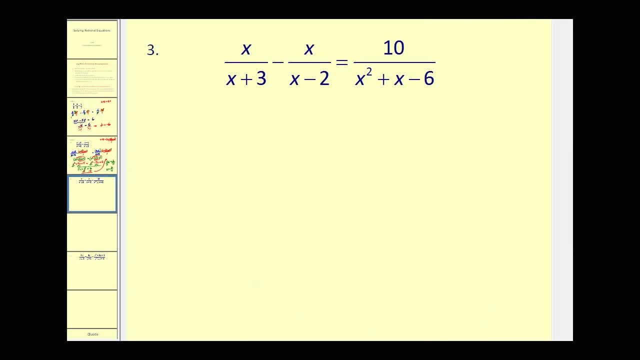 Let's go ahead and try another one. Okay, on this problem we are going to have to factor the denominators to determine the LCD. Let's go ahead and factor this denominator here: The factors of negative six that add to positive one. that would be positive three and negative two. 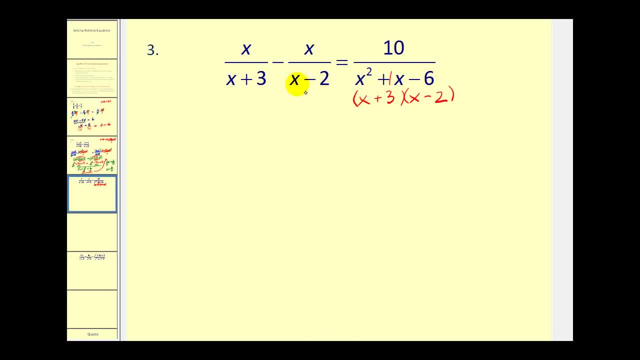 are the same factors we see here. That's what we see in these denominators. So the LCD would be x plus three times x minus two. So we need to multiply each term in this equation by x plus three times x minus two, all over one. 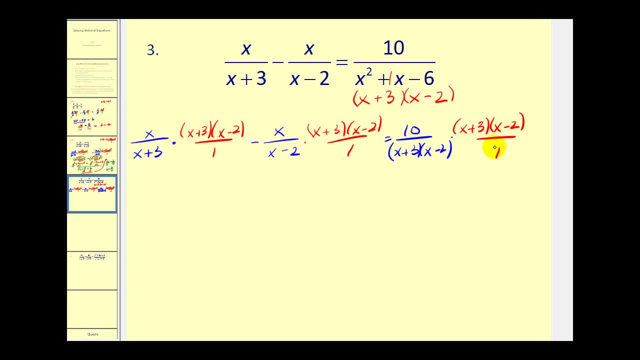 Let's go ahead and do that. So notice, in blue I have the original rational expressions. I did write the right side in factored form And then in red, I've multiplied every term by the LCD over one. Let's go ahead and simplify before we find these products. 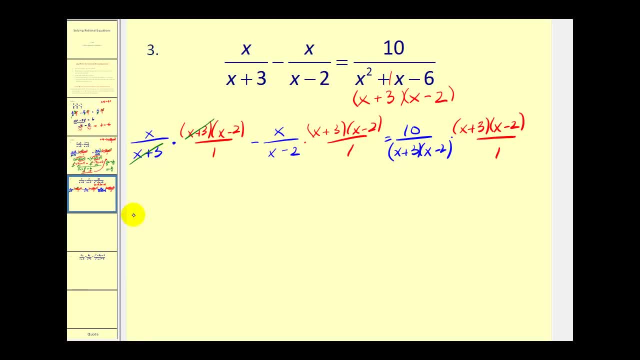 Notice, we have an x plus three and an x plus three, So we're left with x times x minus two. On the next product, we have x minus two on top, x minus two on the bottom, So we're left with minus x times x plus three: equals. 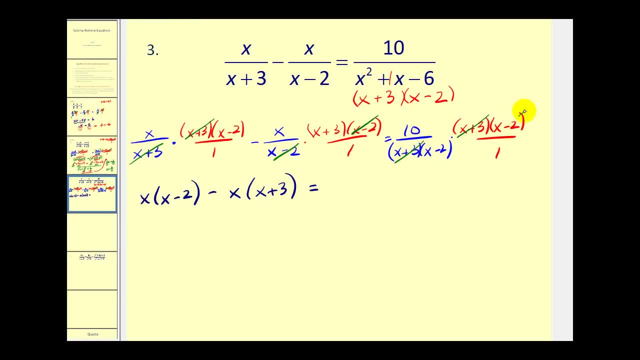 and on the right side, notice- we have x plus three, x plus three, x minus two, x minus two. So we're left with just 10 on the right side. So let's go ahead and solve this resulting equation. So we'll distribute and then solve for x. 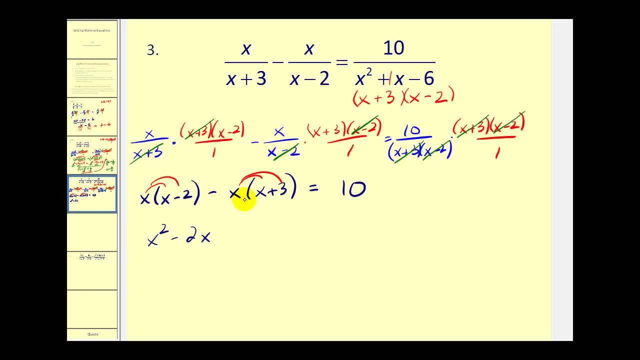 So we have x squared minus two, x minus x. squared minus three, x equals 10.. Notice the x squared terms. simplify out. We're left with negative five x equals 10.. Dividing by negative five X equals negative two. Again, this will be a solution. 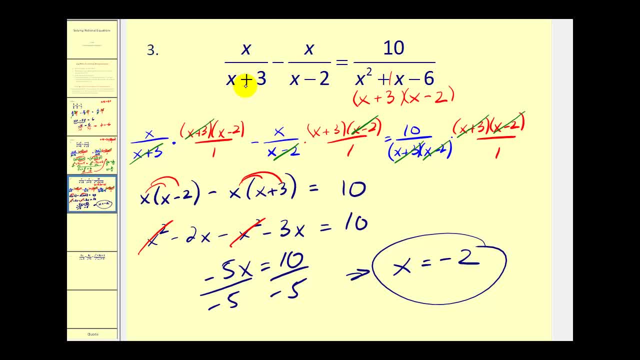 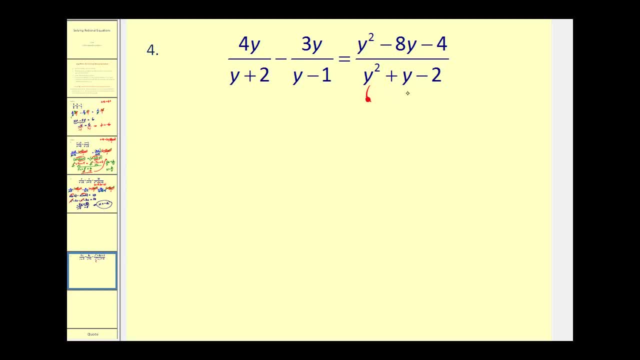 If the solution came out to be a positive two or a negative three, we would have to exclude it. Let's go ahead and try one more Again. we're going to have to factor this denominator to determine the LCD, The factors of negative two that add to a positive one. 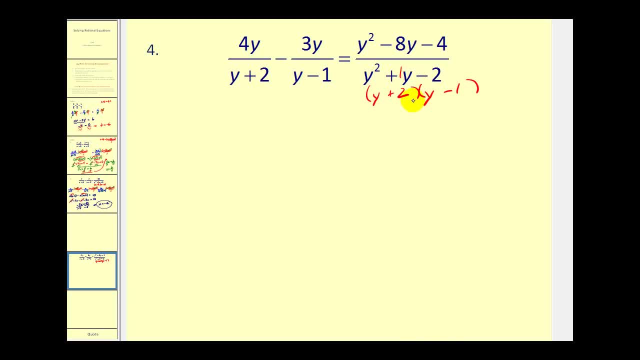 that would be plus two and minus one. So looking at the factors of the denominators, we can see the LCD would be y plus two times y minus one. So we'll multiply each rational expression by the LCD over one. Again in blue we have the original rational expressions. 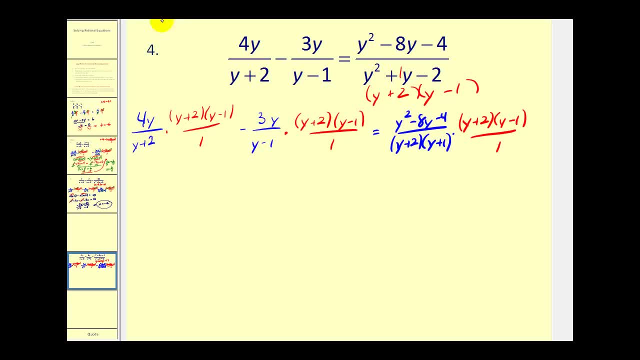 and then in red, we have the LCD over one. Now we'll find each product, but we'll simplify first. So we have y plus two over y plus two. So we're left with four y times y minus one. minus. Here we have a y minus one and a y minus one.